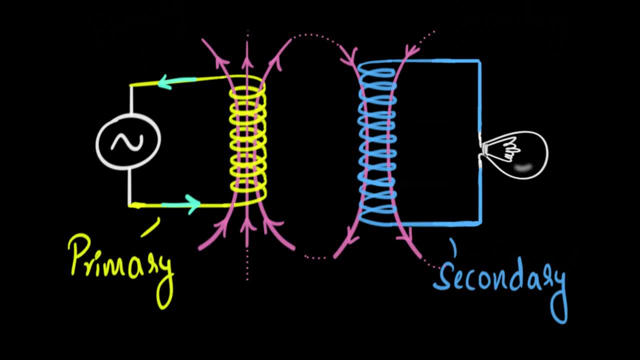 And as a result, as the flux changes over here, as the magnetic field changes over there, the flux also changes in the secondary And again an induction takes place in the secondary and because of that there'll be an EMF generated. 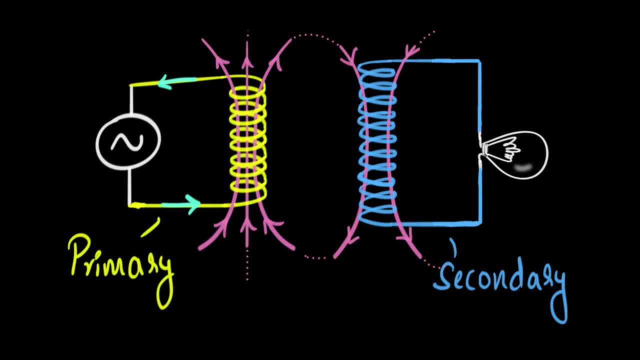 in the secondary and, as a result, there will be a current generated in the secondary, And that's how the bulb starts glowing. Now, at this point you might say: hold on a second. what a waste of time. Why can't I just directly connect the supply to the bulb? 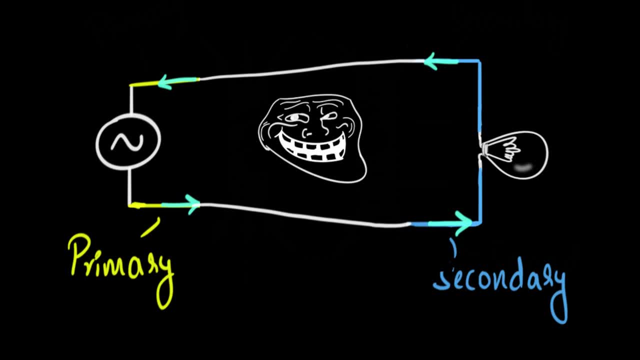 Wouldn't that be just easier? Well, if you do that, then the voltage at the bulb will be exactly the same as the voltage that you are providing over here, And that's not what we want. We want to be able to either increase this voltage. 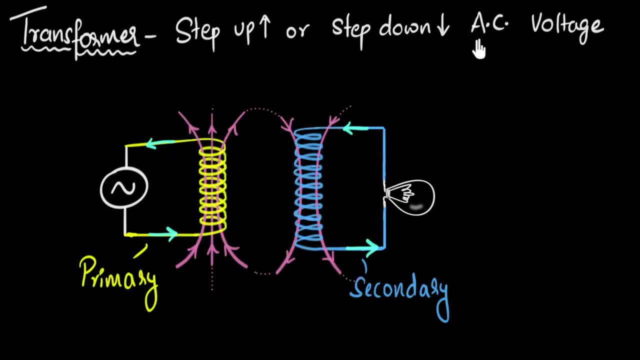 or decrease the voltage, And that's the idea behind a transformer: either step it up or step it down. So how do these coils help do that? Well, let's analyze this. We have the voltages at the primary and the secondary. 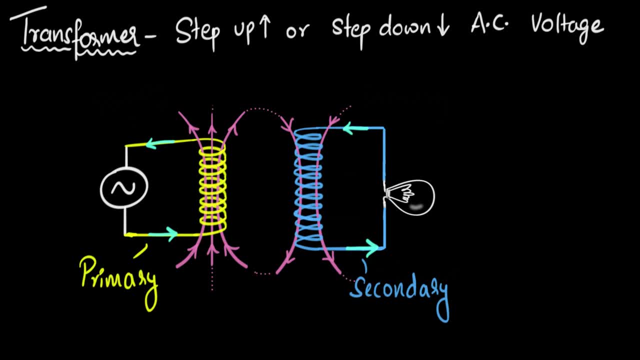 To do that, let's start by looking at a single coil over here. We know from Faraday's law that the EMF induced in any coil due to the changes in the flux is given by E if EMF E is the negative rate of change. 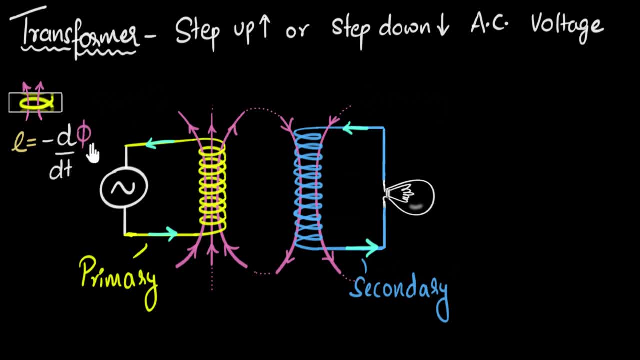 of the magnetic flux. It basically means if the flux changes very fast, then there'll be a higher EMF induced. That's the whole idea behind this. So this is the EMF generated in one coil. Now if there are total, I don't know. 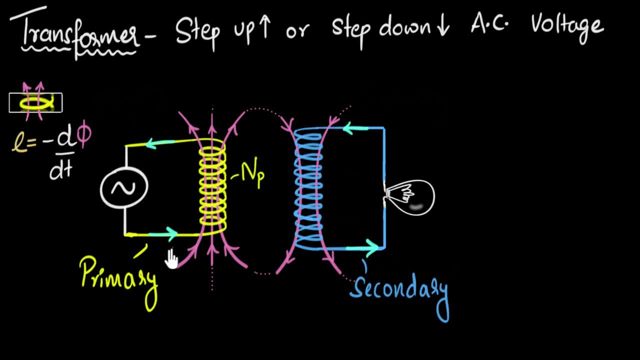 let's say Np, number of coils, where P stands for primary. then what is the total EMF generated? Well, the total EMF generated, that will be the voltage in the primary. That will be just Np times E, Np times E. 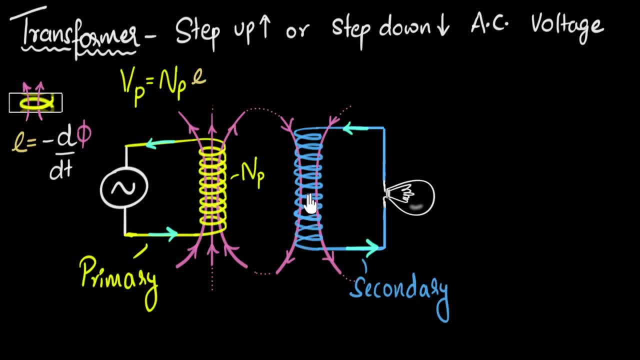 What about the secondary coil? Well, we can do that. We can do similar calculation. We can say that through each coil the EMF generated must be the same. We can, because the flux here and the flux here must be the same. 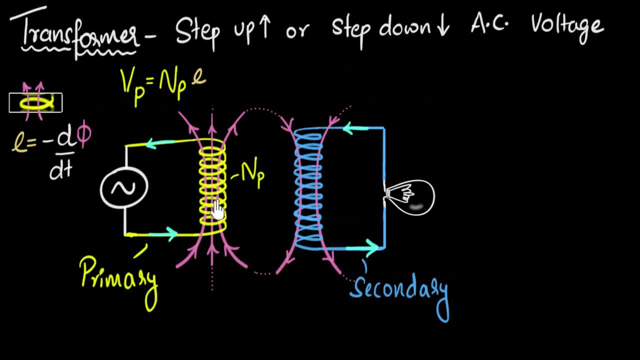 And you might say at this point: hold on. wouldn't the flux decrease because we're going farther away? Wouldn't the magnetic field lines go farther away and become weaker? You're right, but there is a way in which we can make sure. 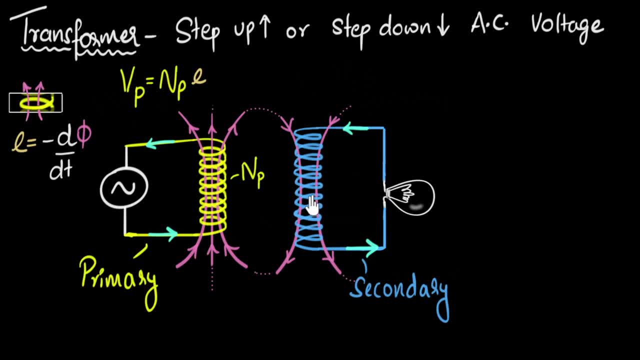 that the magnetic field lines over here and the magnetic field lines over here have the same strength, And we'll talk a little bit about how that happens a little bit later, how we can make sure of that. But if we assume that the flux here is exactly the same, 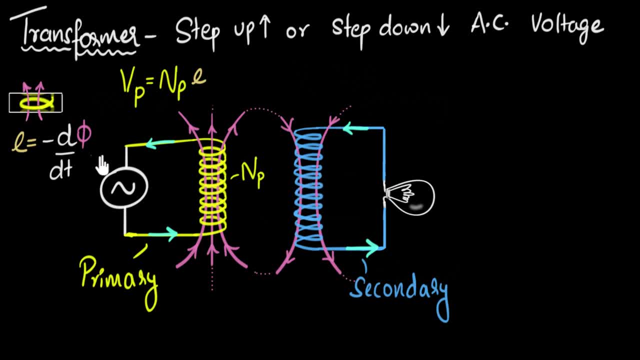 as the flux here at any moment, then the flux through each coil, the EMF through each coil, sorry, is gonna be E, And from that we can now figure out what the secondary voltage is going to be. I want you to pause the video at this point. 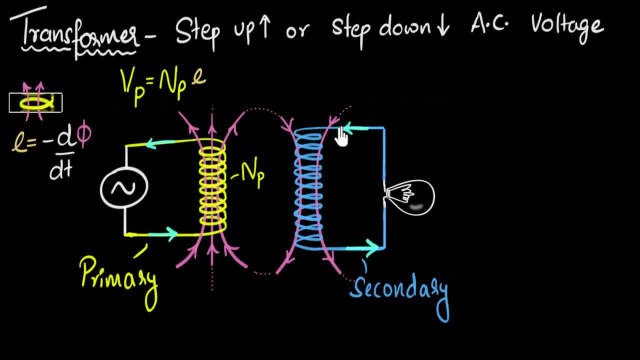 and see if you can, using that, figure out a relationship between the primary voltage and secondary voltage. Go ahead, give it a try. All right, If the number of turns in the secondary is, let's call that as ns, where s stands for secondary. 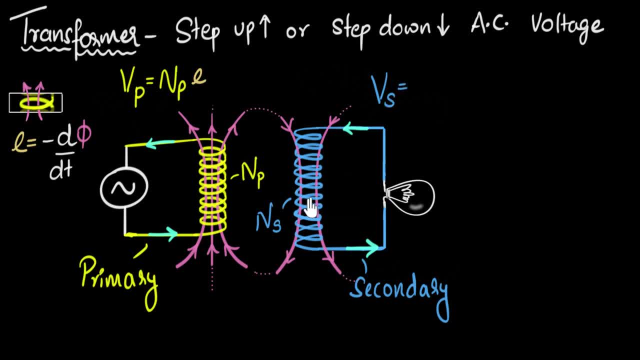 then the voltage in the secondary is going to be well. one coil has emf e ns. number of coils will have ns times e Notice the voltages in the secondary and primary are not the same. If I divide them we'll get the relationship between them. 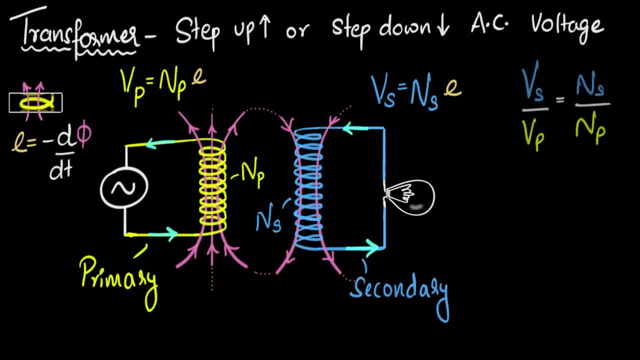 We get: vs divided by vp equals ns divided by np. This means that if the number of turns in the secondary is more than the number of turns in the primary, like shown over here, then notice, the voltage in the secondary would be higher than the voltage of the primary or the voltage of the supply. 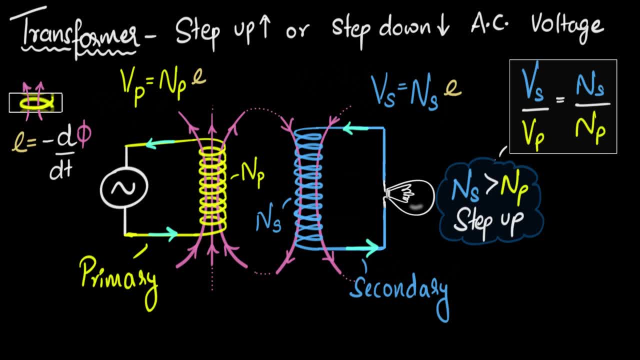 and we call this the step-up transformer, increasing the voltage. That's what happens in your microwaves. Your microwave oven requires thousands of volts to run, but you might know that our AC mains supplies only about 230 volts, so roughly around 200 volts, let's say. 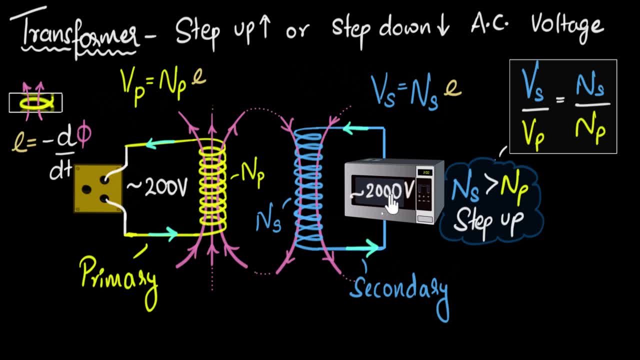 So if you want to increase the voltage, say by 10 times as an example, then all you have to do is make sure that the number of turns in the secondary is 10 times more than the number of turns in the primary. Step-up transformer. 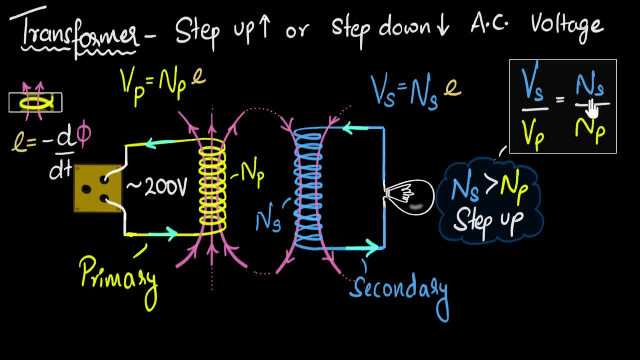 On the other hand, if the number of turns in the secondary is smaller than the number of turns in the primary notice, the voltage in the secondary would be smaller than the supply voltage or the voltage in the primary. we get step-down transformer. 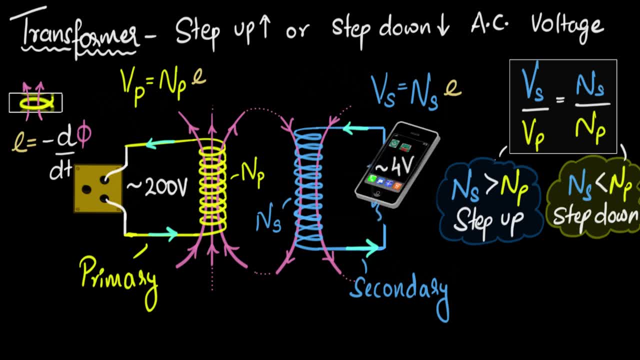 And that's what you would use if you wanted to charge your mobile phone, because it requires a very tiny voltage. The AC supply gives you a lot, so you step it down appropriately by reducing the number of turns And as a bonus notice. 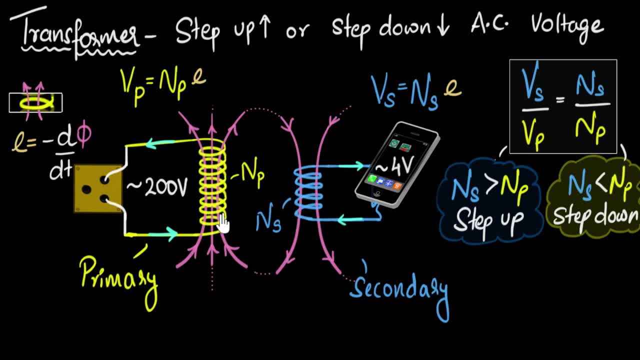 we're able to charge your electric phones without having a direct connection between these two circuits: Wireless charging. That's right. that's how wireless charging works. The secondary coil would be inside the phone. the primary will be connected to your. it would be inside the charging pad. 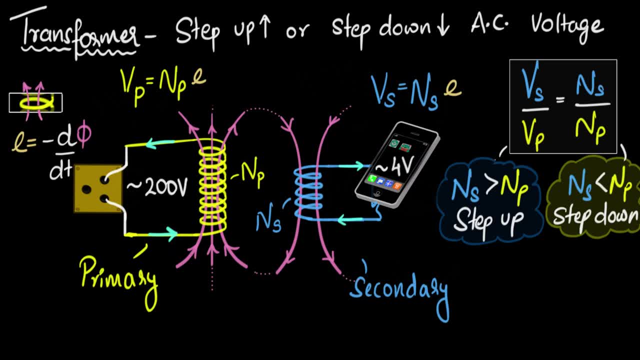 you keep the phone on the charging pad. wireless charging- Beautiful. right Before we wrap up, we still have to answer. how do I make sure that the flux here and here remains exactly the same right Now? before I do that, 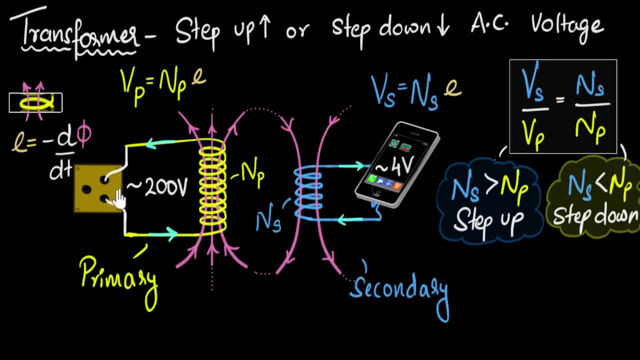 I have one question for you. Do you think this transformer would work on a DC supply? What if I used a battery here instead of AC? What do you think Would a transformer work? Pause and think about this. All right, hopefully you've tried. 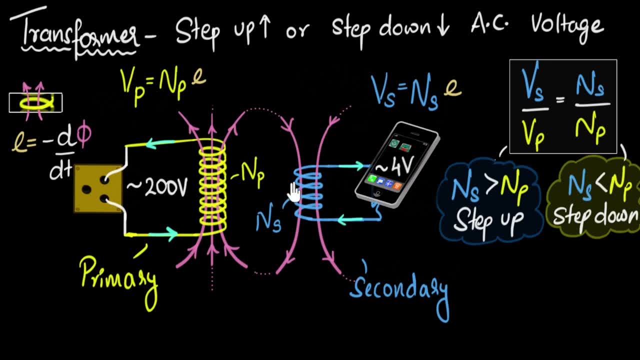 So does it work on DC? Well, let's see. The main principle is electromagnetic induction, And for induction to happen, the flux needs to keep changing, And that can only happen if the current keeps changing. And that does not happen in DC. 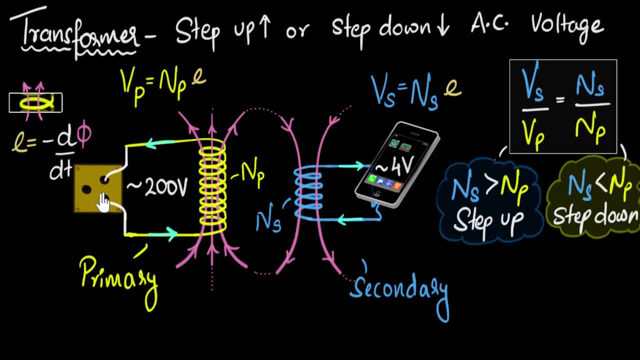 And that's why you cannot use transformers for DC. You can only use it for AC. Okay, lastly, how do we make sure the flux here and here remains exactly the same? Otherwise the equation won't work Well. a way to do that is by introducing: 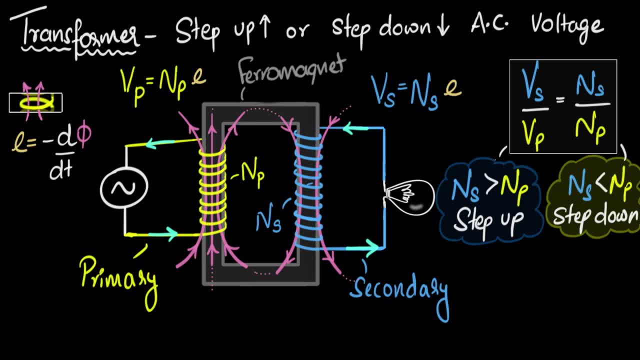 a ferromagnetic core. A ferromagnet has the ability to sort of suck in magnetic field lines And, as a result, almost all the field lines from the primary passes through the secondary, making sure the flux through each coil is exactly the same. 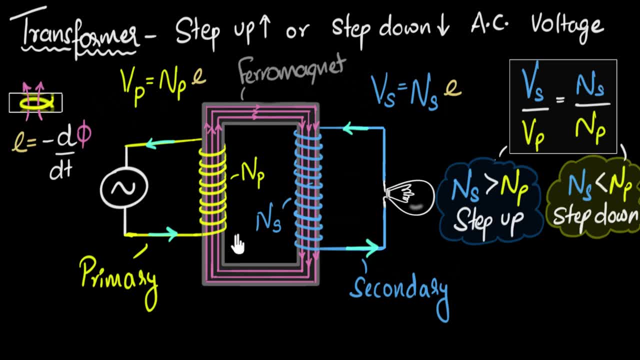 Of course, in a real transformer there will be some flux leakage and the equation will not be valid. But for our purposes we can assume ideal transformers and work with it. And we've just touched the basics. We still have to dig deeper and think about.